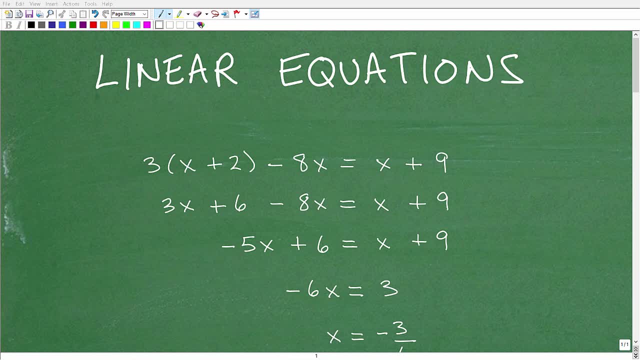 Okay, let's talk about linear equations. So what I want to do in this video is just quickly go over an example problem and just kind of strengthen your understanding on what is a linear equation, okay, what they are in algebra. And this is an example, obviously, of a linear equation, but there's other ways we need to think about linear equations as well. It's a big topic, again, in algebra. But before we get going, let's talk about linear equations. 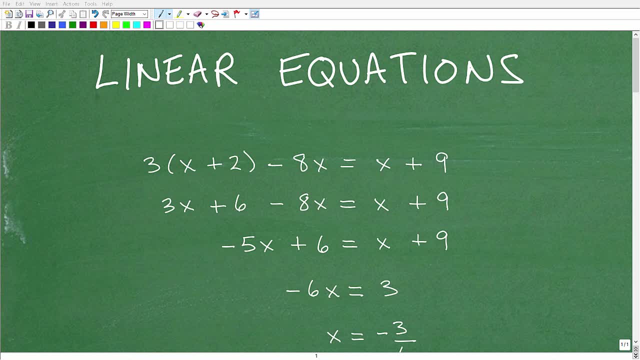 Let me go ahead and introduce myself. My name is John. I'm the founder of Tablet Class Math. I'm also a middle and high school math teacher. And if you're interested in learning from me, I'm going to go ahead and leave a link to my full and complete math courses in the description of this video. But with that being said, let's go ahead and get into a linear equation. So first things first, we got this description. So we have two words here, linear, and then we have equations. So let's just look at this word here, equations. So equations, anything in mathematics and algebra or any other type of mathematics that has an equal sign in it, we describe it as an equation. Okay, so that's the first thing, right? So we have some sort of equation, so it's going to have to have an equal sign. And then here, a linear, if you look at this word carefully, we have this little sub word, and that is line. Okay, so 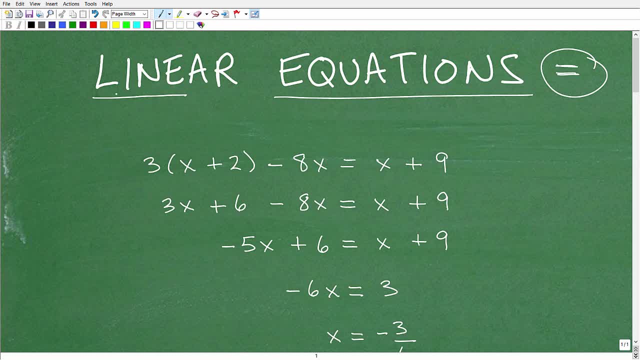 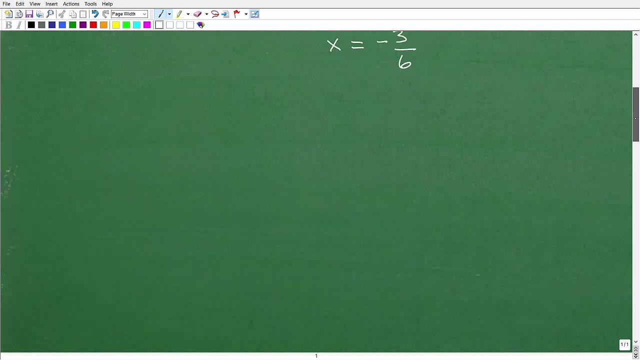 what we're really talking about are equations of line or line equations. Alright, so an easy way to understand it is all linear equations, you can model as some sort of line. So let's go ahead and take a look at this little bit further before we get into this example. Okay. Alright, so let's say we have the xy plane here, okay? Alright, so we have x and we have y. Okay, so line, we're going to have the can look like this they can have some sort of slope all right and the equation 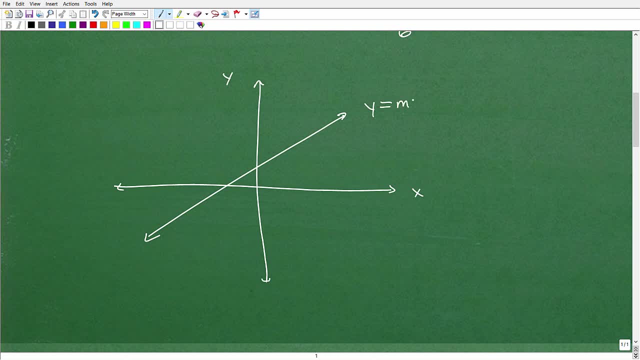 to this line would be something like a y equals mx plus B all right this is called slope intercept so for example this line could be like y equals 2x plus 3 something like that okay now there is another form called standard form okay now it looks like this let's say 3x plus 4y equals 7 that's another form of a line okay or an equation of a line so this is an example of a linear equation and this is an example of linear equation and for those of you out there who've studied algebra before y equals mx plus B is a format that we like to graph lines okay so we're graphing lines on xy plane what we're really doing is you're going to be able to graph lines on xy plane and you're going to be able to 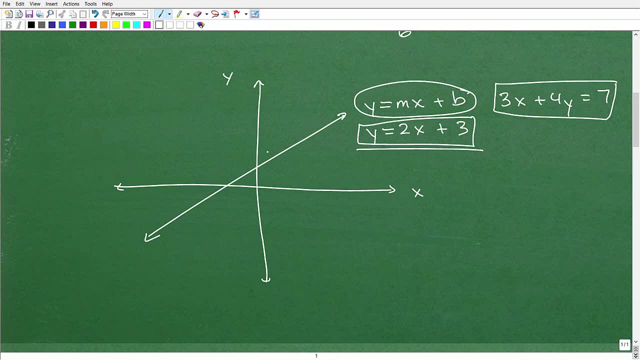 is graphing a linear equation all right and the equation of this line okay is 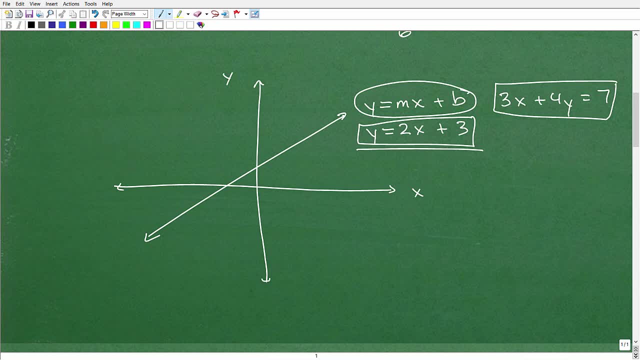 some sort of algebraic equation involves of y and x okay now you can also have lines that go this way horizontal all right these are y equal lines some y equals some number and then we also have lines that go vertical and this is some x equals number okay so for example x equals negative 7 is an equation of a vertical line that goes through negative 7 on the x axis okay so our y equals negative 3 is a horizontal line that goes through negative 3 on the y axis now i don't want to go 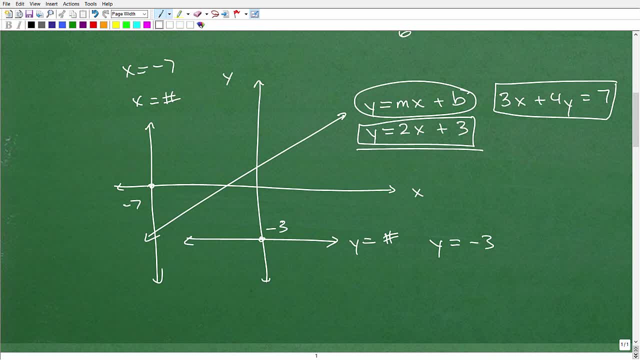 too far in here because again linear equations it's a big topic and it covers that description covers a lot of different type of equations in algebra but let's just make sure you understand linear equations okay or equations that go through negative 7 on the x axis okay so y equals negative 7 on the y axis okay so we're going to have a linear equation of lines right so if i wanted to know what the equation of a line that's a sloped line it's going to involve both the y and x okay so any line that involves y and x is going to be some sort of line with the slope and then here we have our horizontal and vertical lines okay so that's one 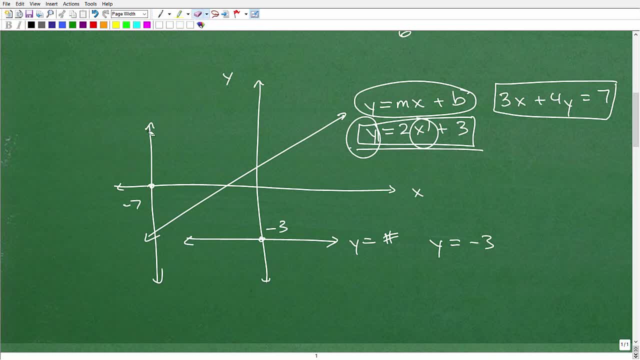 major way to think of linear equations now let's go back talk about another way to keep 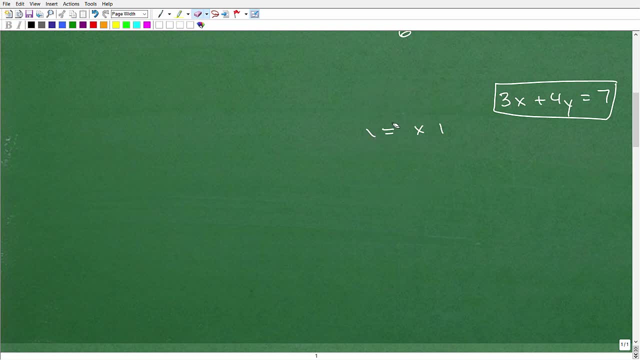 keep , keep your brain straight with linear equations if you will and let's take a look at some example 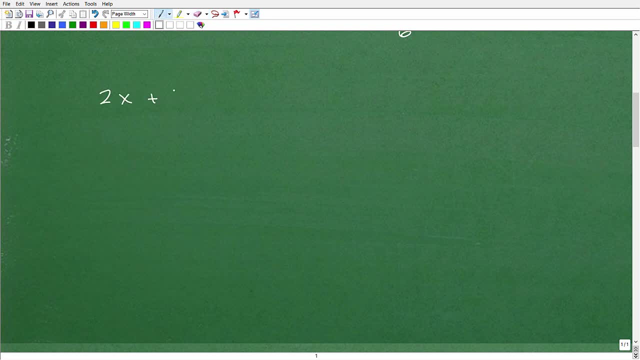 of equations so let's say i have 2x plus 3 equals 9 and let's contrast with this equation with something like this 2x squared plus 3x plus 9 equals 0. okay so this equation over here is linear here all right and this one over here is not i'll tell you what this is in a second 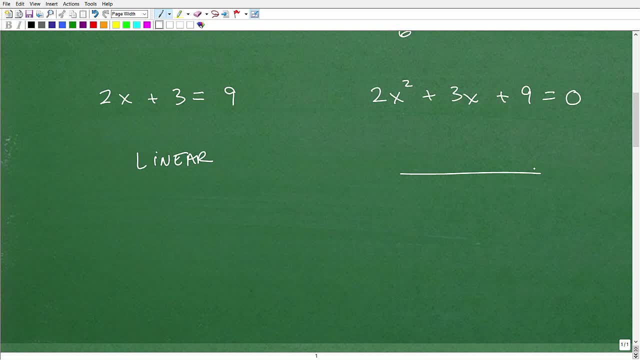 so what makes an equation linear so we know that an equation all right that describes a line okay or the equation of a line is a linear equation but what makes it a linear equation when we look at it algebraically well kind of a simple way to understand this is if you look at the x variable here we have x to the first part of the line our Mat this we so it's another outlier Senior A marking power okay this variable now of course we don't write it to the first power we just write it 2x but really it has a little one up there okay so this is this variable is to the first power unlike this variable here is x squared then we have 3x of course this this is to the first but we don't write it as a first so equations where the highest power is just one and you would see it like this 2x plus 3 equals 9 for example highest power of the variable is just one is a linear equation okay now if we have the highest power to the variable let's say our variable X 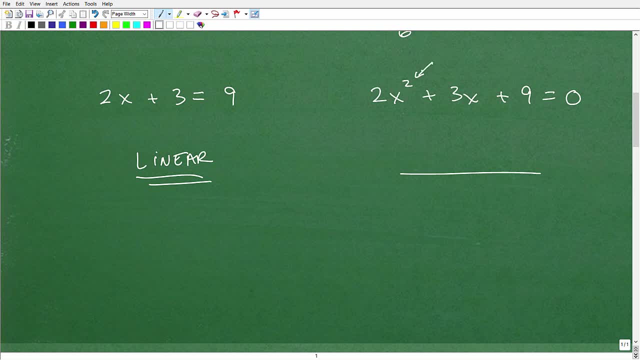 here is 2 okay but go up one we have another type of equation okay this equation is called quadratic okay this type of equation this is a quadratic equation and it has a different shape it has a shape of a parabola 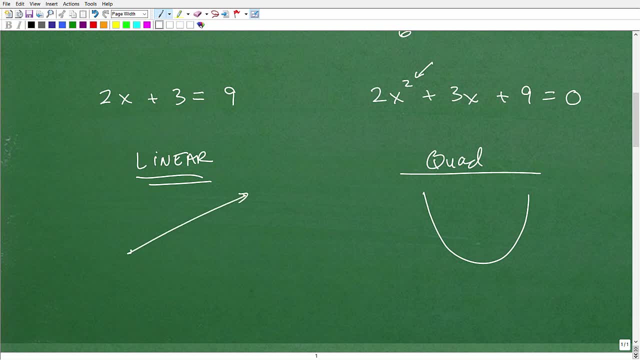 okay here these type of equations have a shape of a line so it's really important that you know when you're using terms like oh we're going to study a linear equations you have a concept of what they are what they are not of course there's other type of equations in algebra many different 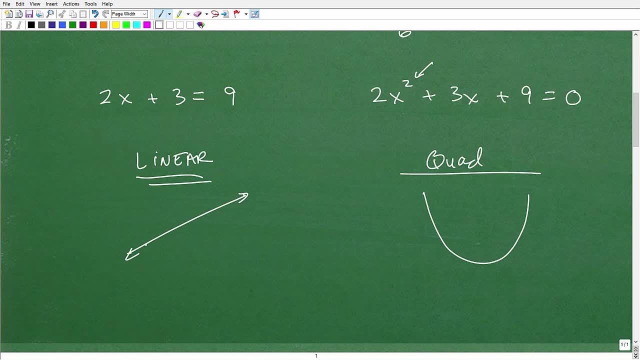 type of rational equations or radical equations systems of equations exponential equations on and on and on so you know these terms you know 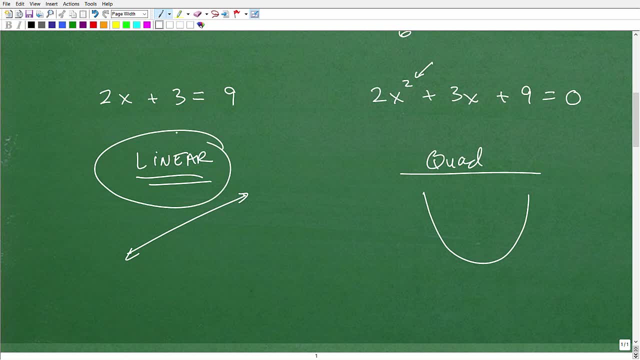 mean something okay so anyways let's focus in again on linear equations now here let's take a look at this 2x plus 3 equals 9 one of the things that you want to be able to do when we're talking about linear equations is to solve them okay how do we solve linear equations this is again fundamental basic algebra stuff and now let's go ahead and take a look at this example 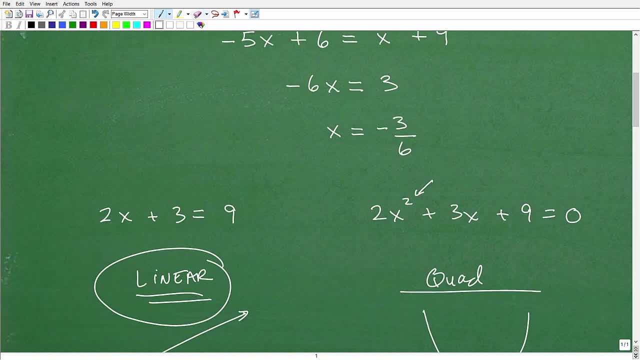 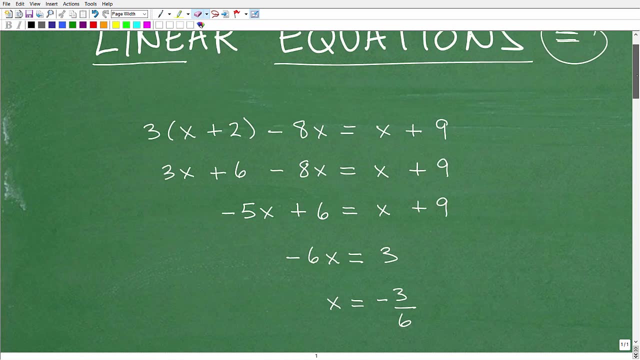 up here let me go ahead and erase this so we don't confuse what's going on all right so let's just go over this quick example of a linear equation and what we're trying to do here 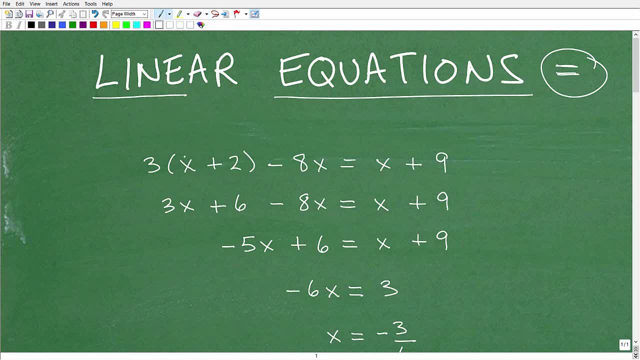 first of all let's just see here we have all x's and it's to the first power okay and there 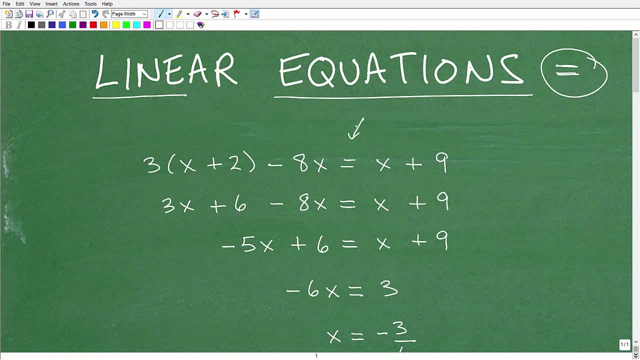 obviously isn't a an equal sign so it is an equation so what we want to do here is to be able to solve for x okay solve this linear equation all right so there's all kinds of different ways to solve linear equations so let's go ahead and take a look at this 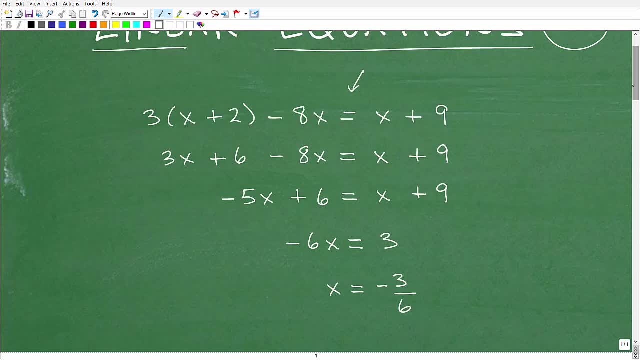 different varieties of linear equations some involve fractions positive negative numbers or decimals let's just take a look at this problem because this will kind of illustrate some of the things you really need to be focusing on when you're dealing with many types of linear equation problems okay so the first thing is the following let me see if i can highlight this well that doesn't work so well but when we're looking at a linear equation okay we're looking at a linear equation and we're looking to solve it what you want to first uh focus in on is anything with parentheses any any expressions like this with parentheses okay so here i have x plus two i have this three outside this x plus two so what we want to do is look to see if there are any of these situations now it could be an uh an x minus two or it could be x minus five uh whatever the case is and there could be multiple different things going on here okay anything with the number outside of a parentheses like this is a signal for us to say hey do the distributive 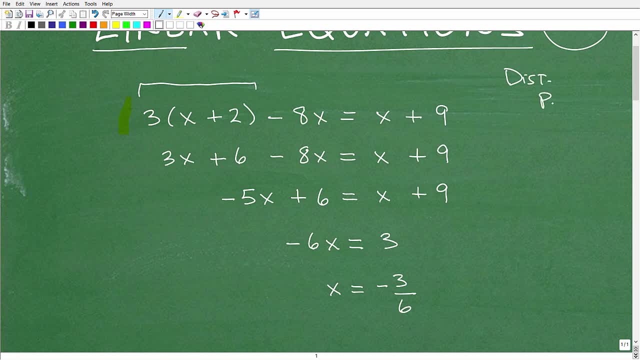 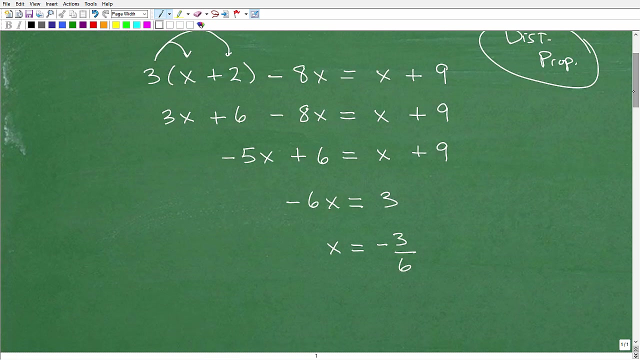 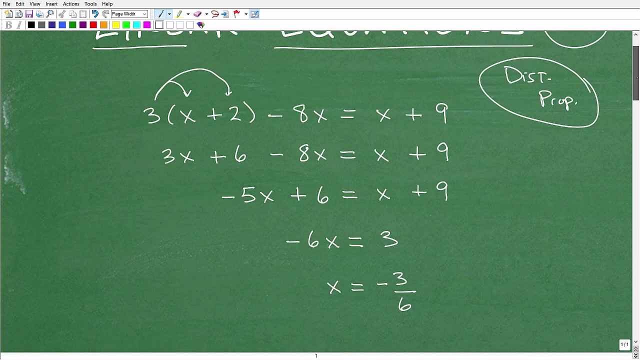 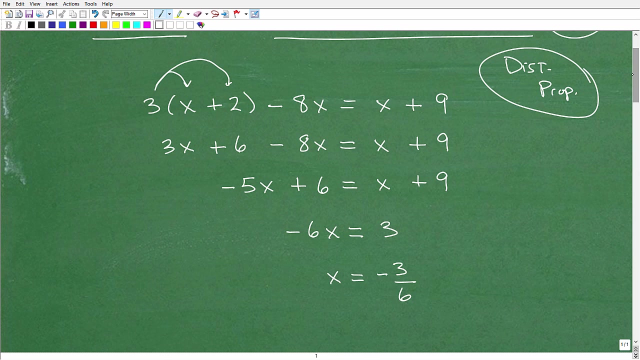 property okay the distributive property okay now i could tell you my years teaching math many many many many years this right here the distributive property so many students mess this up don't let that be you okay you got to make sure you know how to do the distributive property well all right so let's get back to the distributive property so let's get back to the distributive property what is it well that's a whole nother lesson in of itself but basically this value outside of the parentheses the first thing you have to do when you're solving a linear equation is to go ahead and distribute okay this value to our inside uh terms here so it's going to be three times x or three x and then three times is two and that's six okay and then we'll just rewrite the rest of the equation like so okay so the first thing you want to be you want to do is you want to do when you're dealing with linear equations is to look to see if you have any distributive property situations and then go ahead and handle those now there are a couple different other stylistic or different approaches that you could take you could combine like terms etc etc but let's just kind of keep keep it simple and give you kind of a procedure you can always follow because you can't really combine like terms in an equation until you've finished doing the distributive property 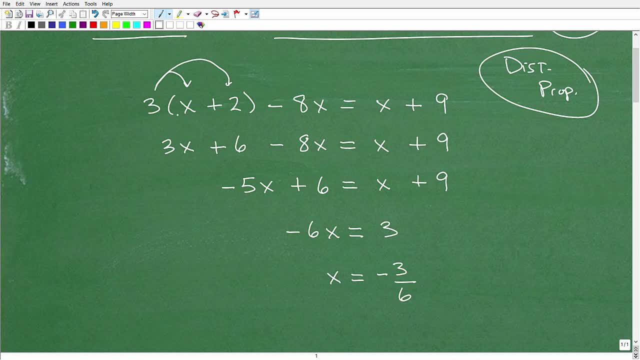 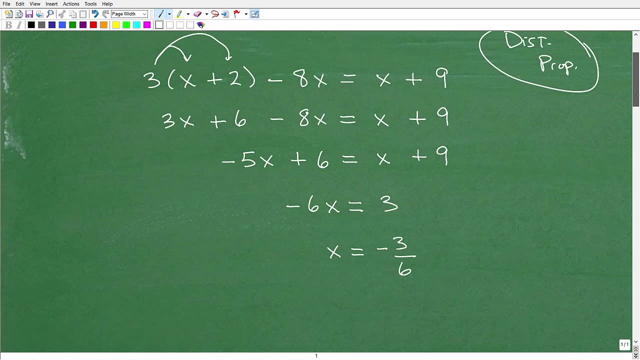 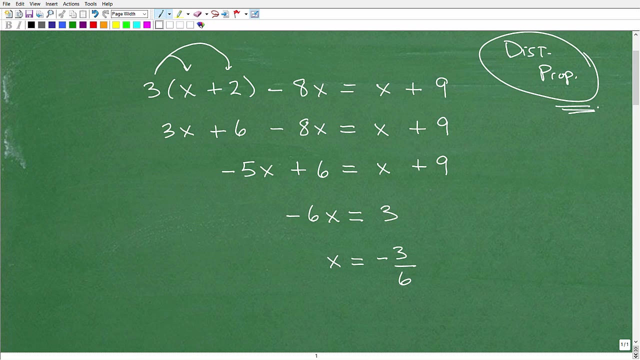 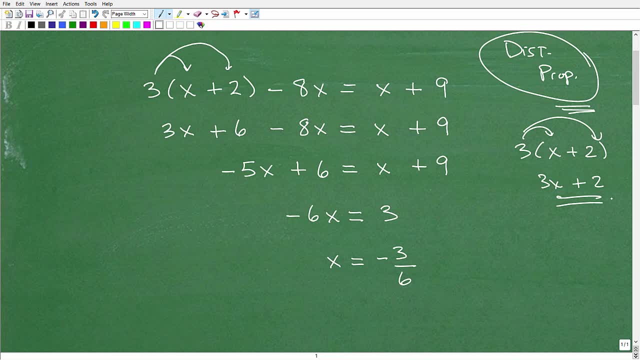 until you really kind of master this so really focus on the distributive property okay so now once the distributive property is done we want to go ahead and combine like terms on both sides of the equation and i'm assuming that you've studied you know the distributive property and like terms again this is just a kind of overall video uh you know i'll do more in depth if you're on my 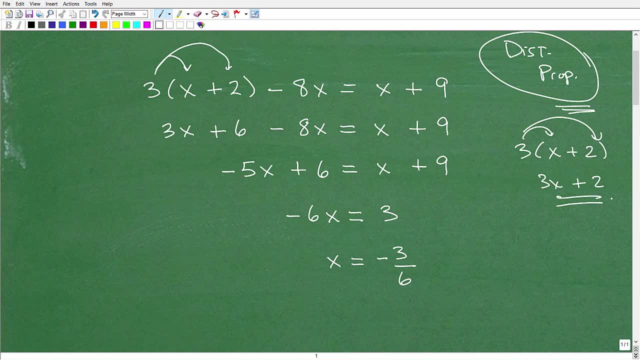 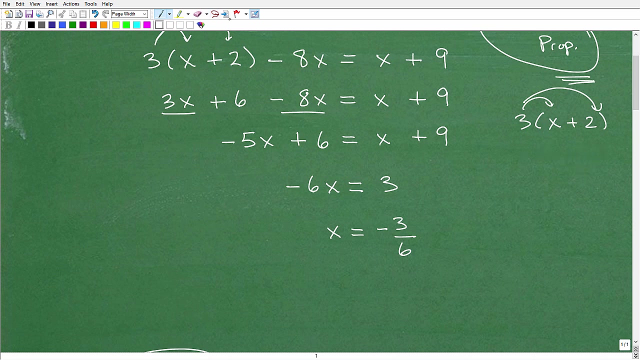 youtube channel i got many many more videos or more in depth on this but combining like terms is focused on the left hand side of the equation so it's like okay 3x and negative 8x okay these are our like terms okay so i can combine them so i just add the coefficients 3 and negative 8 and that gives me negative 5x and then i have my 6 here so i can rewrite all of this or simplify this as negative 5x plus 6 and then on the right hand side of the equation i just have x plus 9 and i can't really simplify that much more than it already is so that leads me to this situation now give ourselves some room all right so here what do i need to do well when you're solving equations remember you want to get all the variables on the left hand side you want to get all the numbers on the right hand side so this is like your next kind of phase of this uh problem okay so let's go ahead and deal with this x so this is really a 1x okay it's on the right hand side i want to move it over to the left hand side so i'm going to subtract a negative 1x here but i have to also do it to the other side of the equation okay so the main idea okay when the main principle when you're solving equations is whatever you do to one side of the equation as long as you do it to the other side you're okay okay you kind of think of this as a teeter-totter all right whatever you do here as long as you do here it it keeps in balance so now you want to 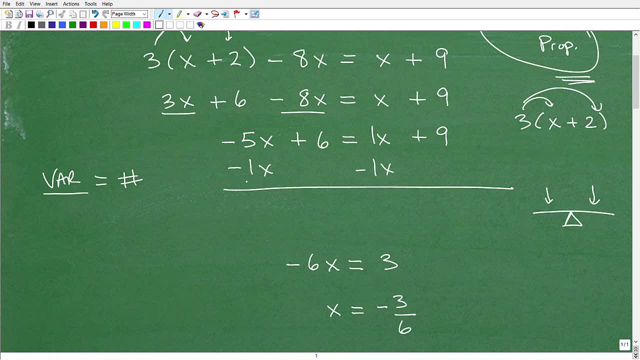 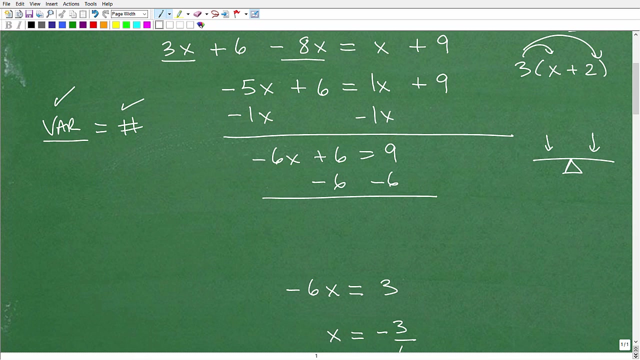 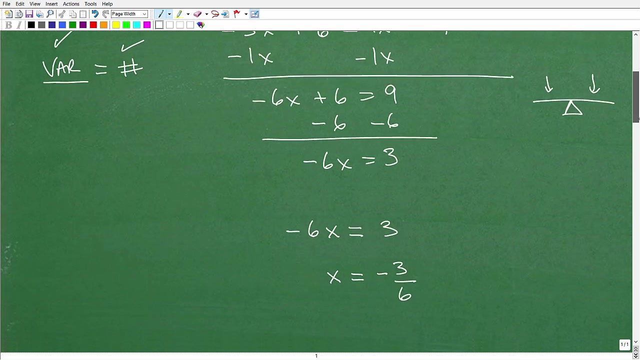 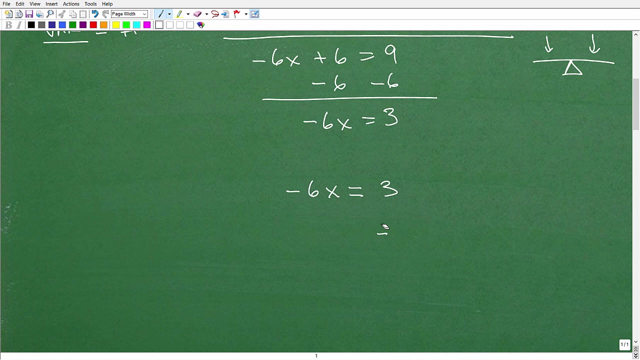 kind of add down and column format so negative 5x plus a negative uh 1x is going to give me this negative 6x plus 6 my x over here went away but really what i did was move it to the left hand side and i have that equal to 9 okay all right so keeping in mind do i have all my variables to the right hand side yes i do but i don't have all my numbers to the right hand side let's go ahead and make that happen now so i'm going to go ahead and subtract 6 okay i'm going to use the same concept from both sides of the equation and that gives me you can see i already did the work in advance but let's go and explain each step it's really important so this give me a negative 6x all right just bring this down the sixes go away okay positive positive 6 plus a negative 6 is 0 and then here this is 3 all right now at this point i i'm left with negative 6x equals 3 so we see our answer is going to be x equals negative 3 over 6 but how do we get to that point and obviously this is actually going to be a negative one half you got to reduce that answer but at this point you're left with a basic what we call one step equation so to solve for x to get x by itself i have to divide both sides of the equation by a negative 6 and that's what this is right here okay so x is going to be equal to 3 divided by negative 6 okay of course when we reduce that that's going to be negative one half and that is the solution 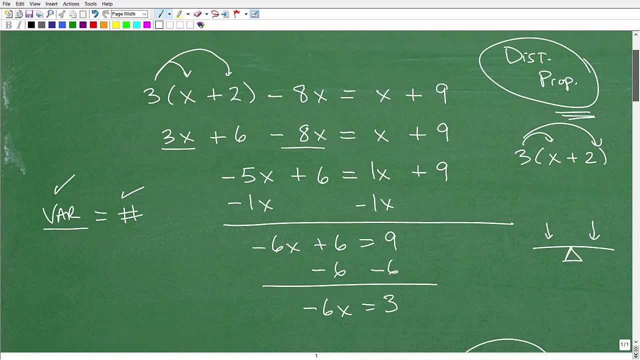 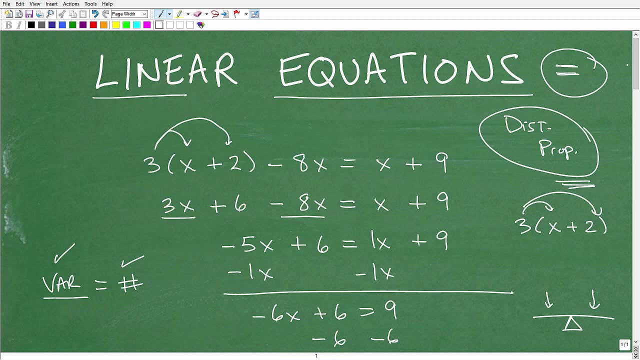 to this particular linear equation right so um this is a real kind of basic problem but it has enough variety in it so enough of the moving parts that are found in a lot of linear equation um examples so here we are solving a linear equation okay but there's other things we could do in this broader topic you could graph the linear equation or you can find the equation of a line which is in itself a linear equation so you want to keep this topic 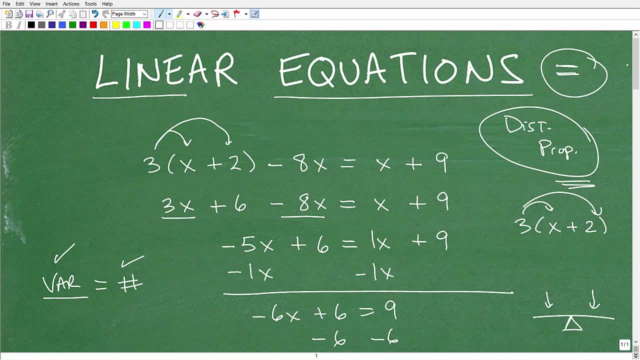 you know keep the description of what you're trying to do You know, you know, don't confuse it. It is a super important topic and it's absolutely critical in your understanding of algebra and whether you're taking another kind of class, like I say, college algebra, algebra two, whatever, even pre-calculus does make a difference. This is stuff that you need to know. And even the most, you know, advanced students, like say you're in, you know, pre-calculus or even calculus, a lot of students don't, you know, don't remember what is, you know, what exactly do these equations mean and, and, you know, the description of them. 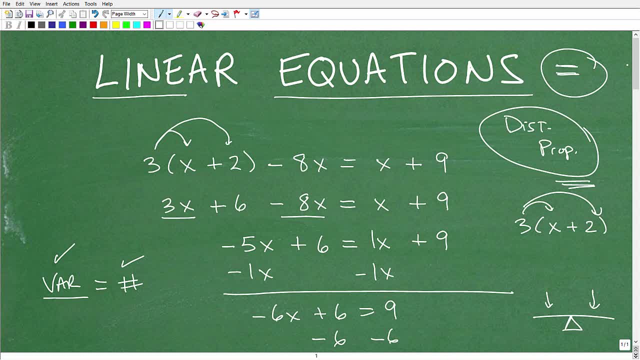 Anyways, I hope this video helped you out to get clearer on what linear equations are. Again, if you want to, you know, realize. 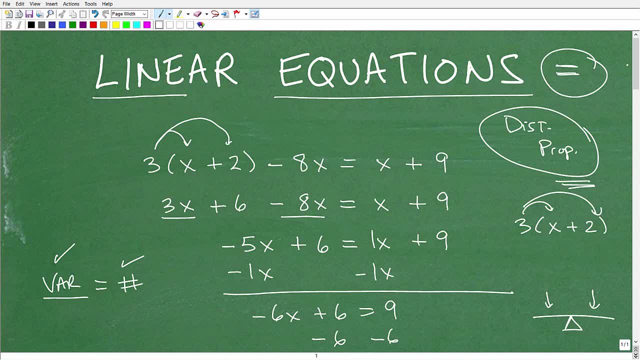 If you want to really learn from, you know, from me in a, you know, really more in-depth manner, I'm going to go ahead and leave a link to my math program in the description of this video. But with that being said, I definitely wish you all the best in your mathematics adventures and, of course, in linear equations. Thank you for your time and have a great day. 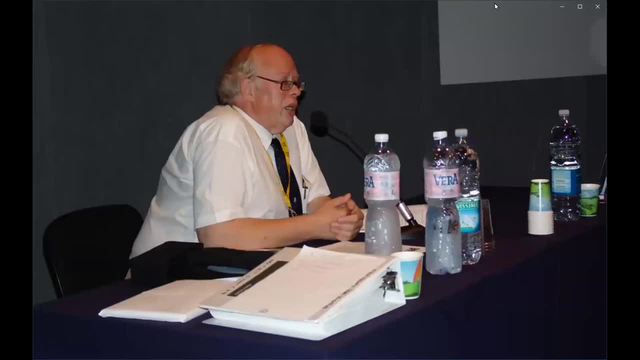 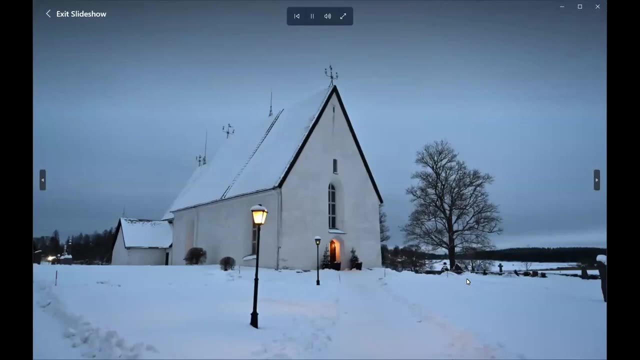 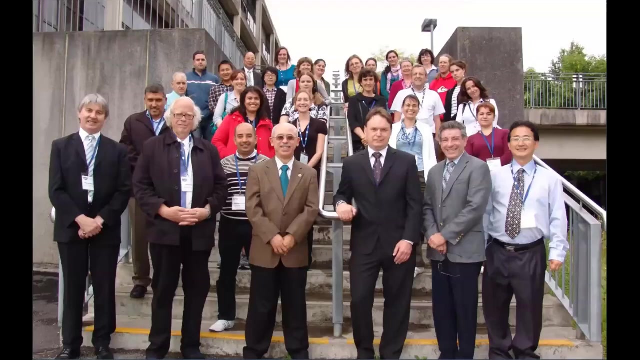 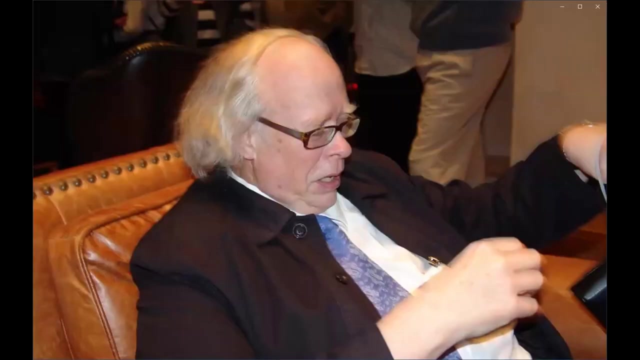 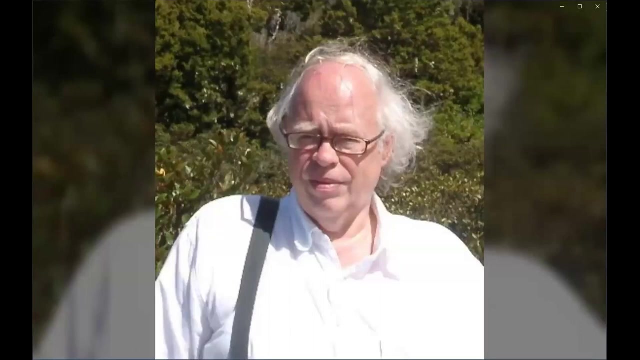 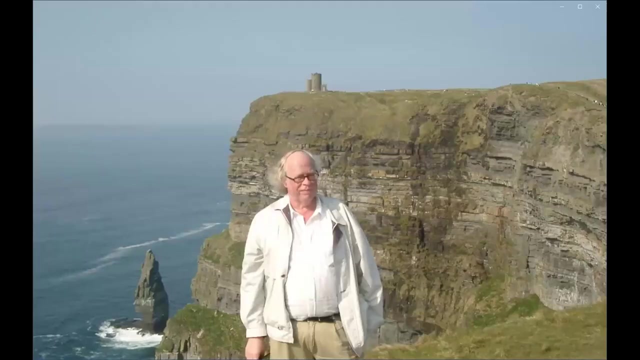 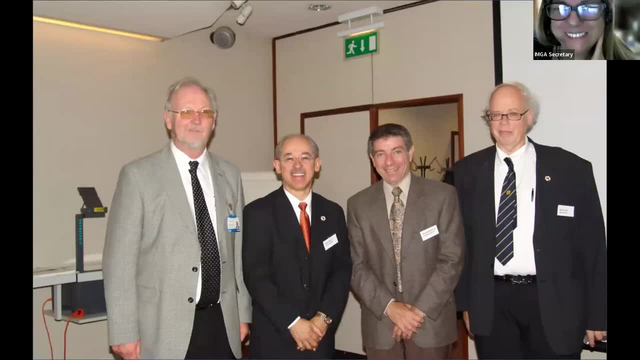 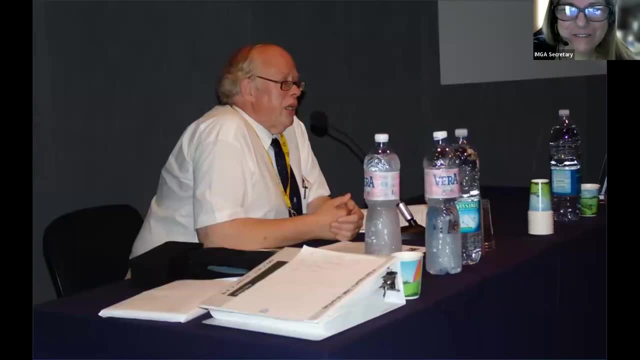 Thank you so much for this important. You are more than welcome. Let me. I cannot. 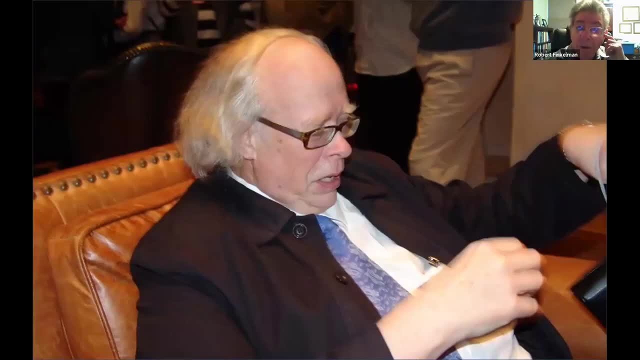 Oh, there's a question. Okay, I have to wait till you give me permission.